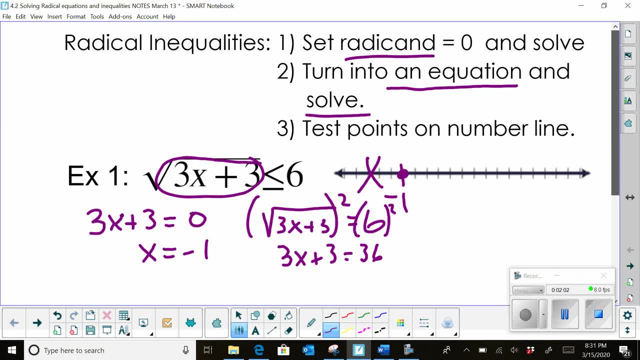 When you solve that equation, you'll subtract 3 and divide by 3. You'll get x equals 11.. So we're going to come over here. I'm not going to really count, I guess I should. Okay, here's 11.. And because it was in less than or equal to, that's a closed circle as well. 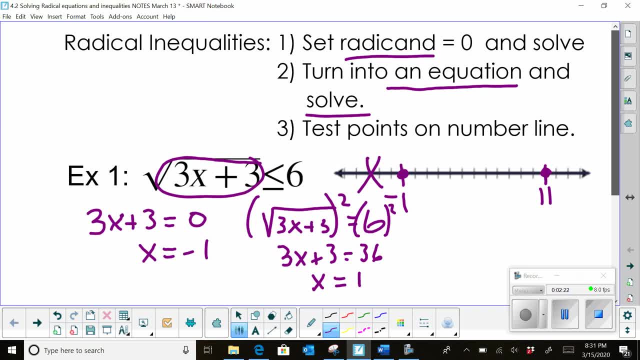 So now we're going to test some values. Well, something easy to test: between negative 11 and 1 is 0. If I plug in 0 into the inequality, I get the square root of 3, times 0, plus 3, is less than or equal to 6.. Well, that's. 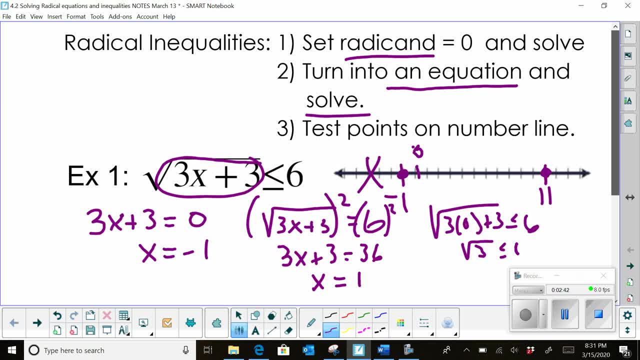 the square root of 3.. It's less than or equal to 6,, so that's true. Sorry, So that's true. we're going to shade in that part of our number line If I plug in a number greater than 12-. 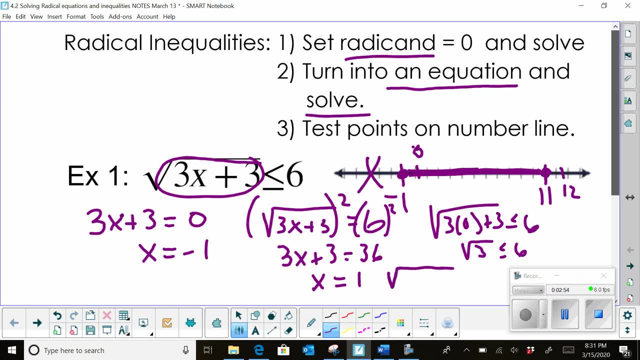 at 11, like 12, that's going to give me the square root of 3 times 12, plus 2,. 3 is less than or equal to 6.. Well, 3 times 12 plus 3 is 39. And the square root of 39 cannot. 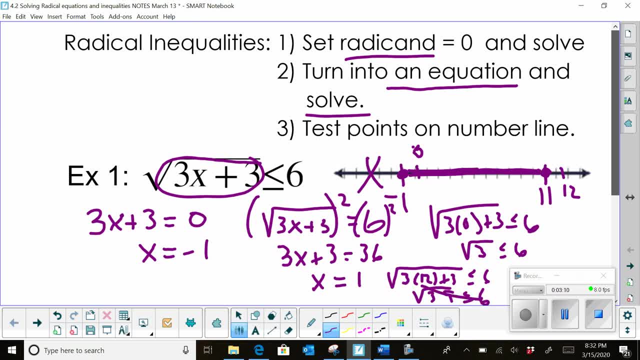 be less than or equal to 6, because that would be the square root of 36.. So that's false. So our solution is from negative 1 to 11, including those points. So my solution is going to be bracket negative 1, comma 11.. And that's the solution. So that's our first example. 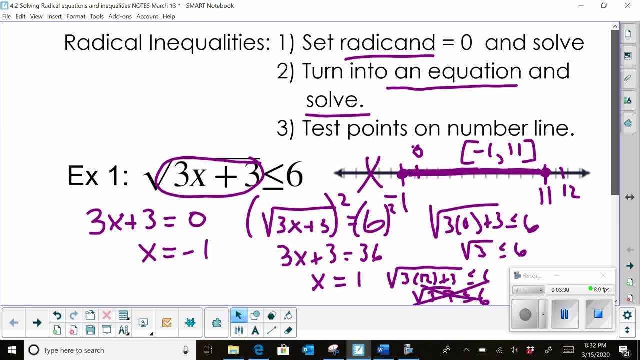 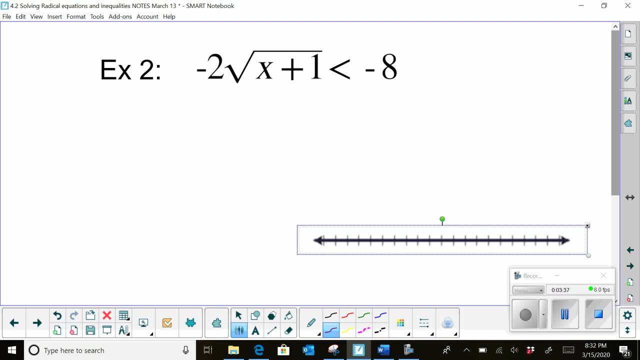 Let's move on to the next example. We're going to do this one, which is the square root of- I'm sorry, negative 2. square root of x plus 1 is less than negative 8.. On this one, you'll notice that the radical is not isolated. We've got to get the radical isolated. 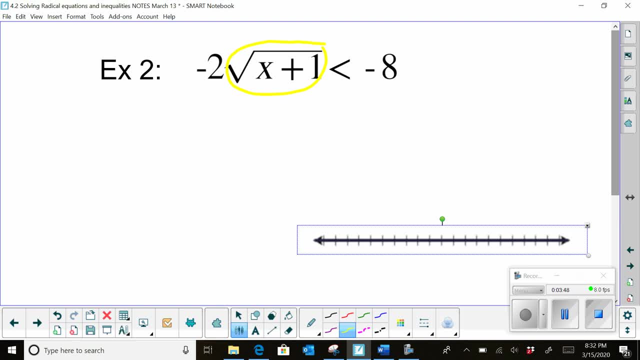 when we turn it into an equation. The first part is no different than the last example. You're going to take your radicand x plus 1 and set it equal to 0. You get x equals negative 1.. So again we know x can't be anything less than negative. 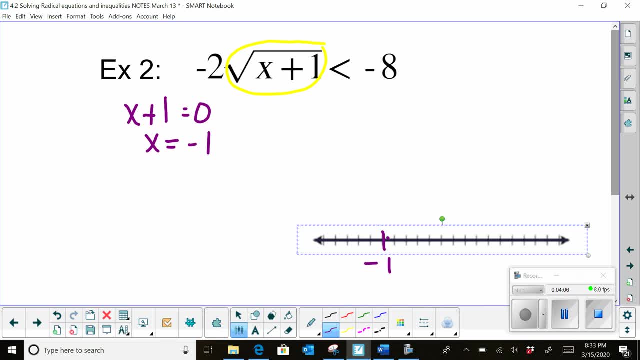 1, because that would give us a negative under the radical. So that's going to be a closed circle, because we get equal negative 1.. That's okay, but nothing less. So we don't even have to consider that part of the number line When we make it into an equation. we're going 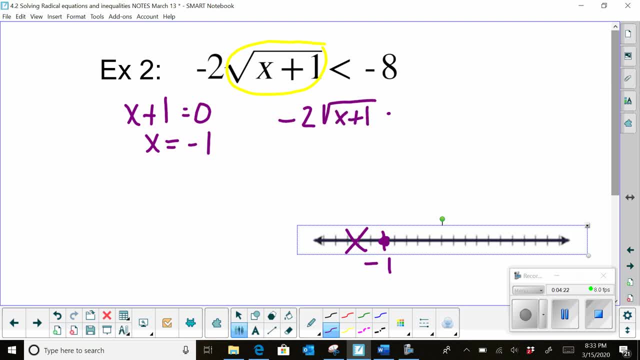 to make it equal to, instead of less than So, we're going to divide both sides. We're going to do this by negative 2. first, Remember, we have to divide. You're going to get the square root of x plus 1 equals 4.. Sorry, my plus sign isn't very good. And then you're 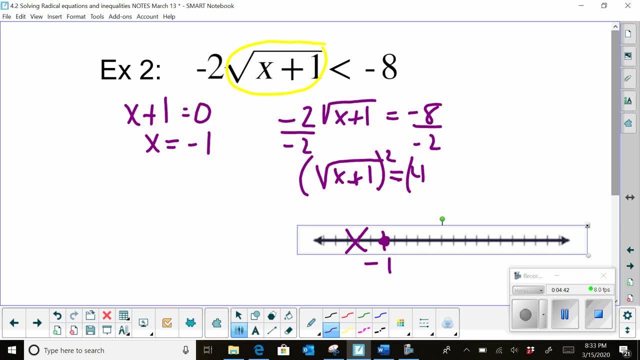 going to square both sides. So you're going to square both sides. You get x plus 1 equals 16.. And then subtract 1 on both sides- Sorry, my stylus is acting funny- So you get x equals 0.. Again, we're going to plot that on the number line. We'll just put it over here. 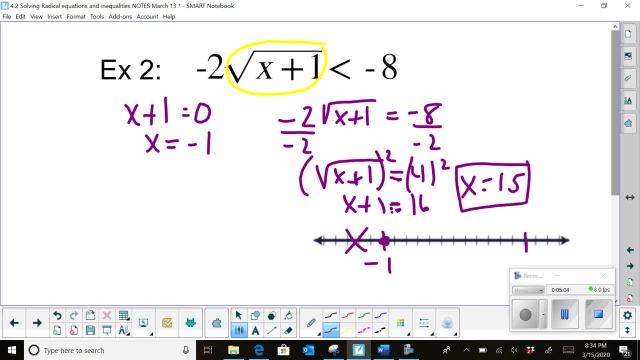 That should be an open circle, because it's really less than not or equal to. So now we can pick some values to test. Again, 0 would probably be a good thing to test. We'll test 0 and maybe 16.. So we're going to come over here. We're going to test 0.. So I'm going 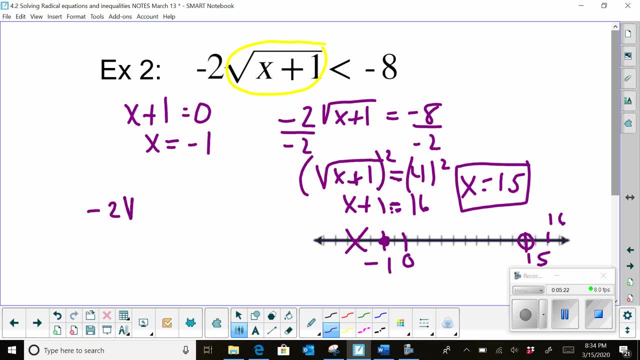 to come to the side, We're going to do: negative 2 equals 0 plus 1.. So we're going to do: negative 1 under the radical is less than negative 8.. So we're going to have negative 2 times. the square root of 1 is negative 2.. Well, negative 2 is not less than negative 8 because 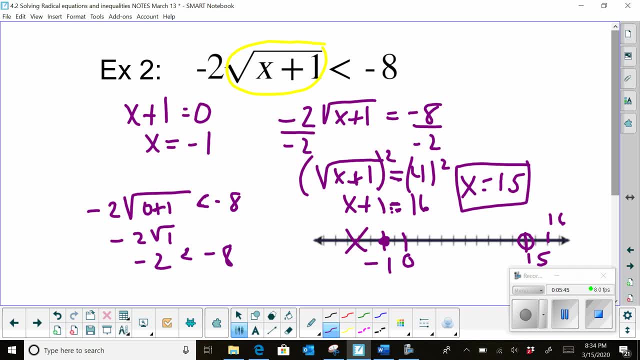 negative 8 is less than negative 2. So that's going to be false. right 0 does not work, So that would be false. Don't shade that part of the number line. And then when I plug in 16, let me scroll down just a little bit- When I plug in 16, I'm going to have negative. 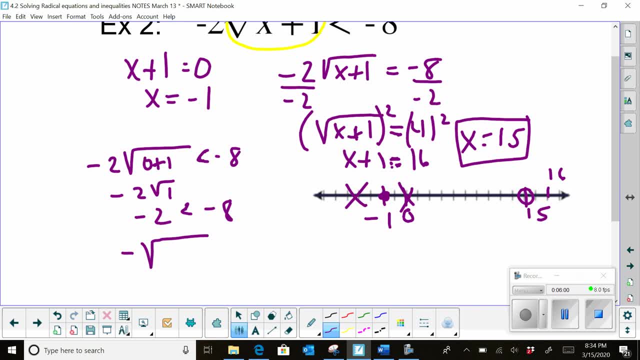 2 times the square root of 16 plus 1 is less than negative 8.. So that's going to be negative 2 times the square root of 17 is less than negative 8.. Well, I know that: negative 2 times. 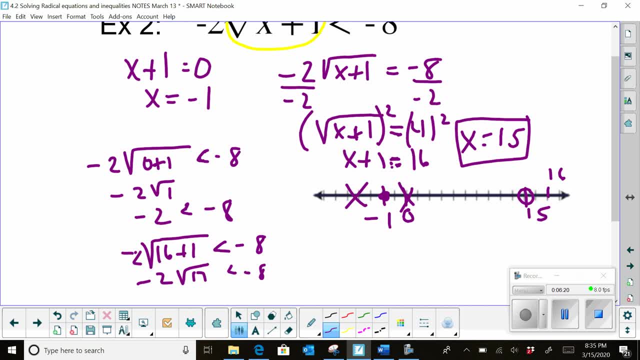 the square root of 17 is going to be negative 2 times, something a little bit bigger than 4.. So that would be less than negative 8. So that checks. So I know I'm going to shade off. So I'm going to shade off to the right, And that's just going to be greater than 15.. You. 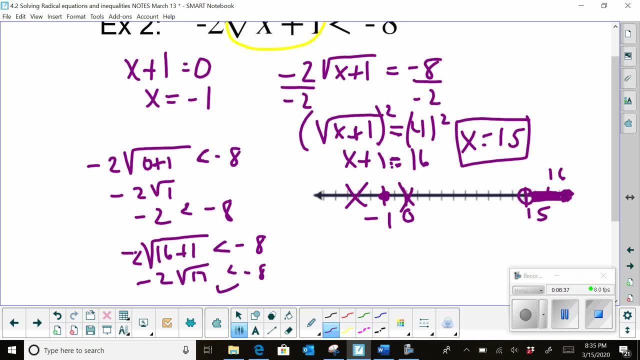 don't care about negative 1, because if nothing to the left of 15 works anyway, then negative 1 doesn't matter. So you're going to do 15 to positive infinity And that would be how you write your answer in interval notation. Hopefully I'm writing well enough for you. 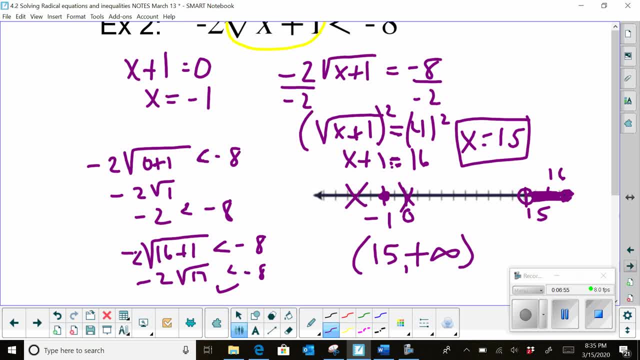 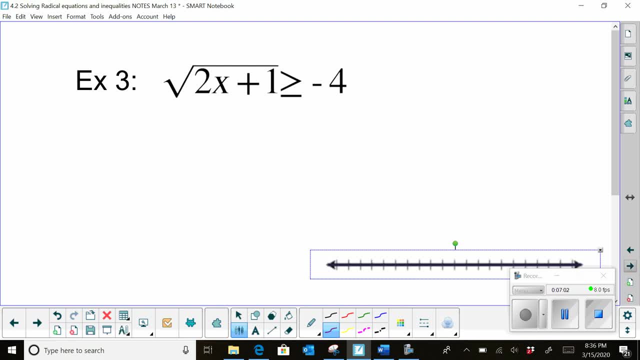 to understand. I'll get better as we go through, I promise. Next example you're going to do: the square root of 2X plus 1 is greater than or equal to negative 4. This time, when we square both sides, it will get rid of the negative. But first again you go to your. 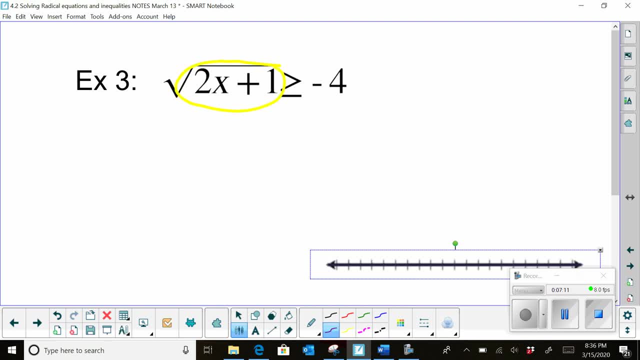 radicand set 2X plus 1 equal to 0. You're going to get X equals negative 1 half. So again, we'll put that over here on the number line, maybe over here kind of on the left. Then when you turn it into an equation, you're going to get a sum of the squared root of 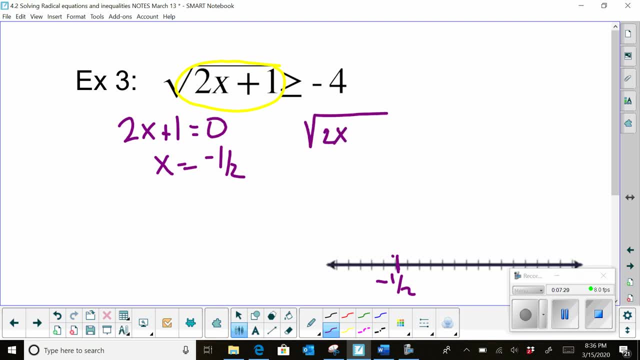 an equation. You're going to square both sides Again. squaring gets rid of the radical. You're going to have 2x plus 1 equals negative 4 squared. It doesn't like my 2.. It's 16.. And 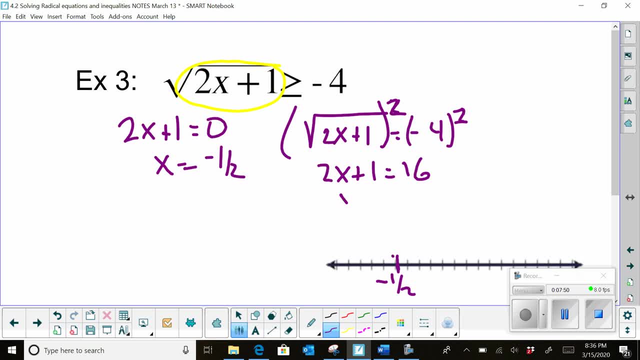 then you're going to solve for x, So you'll get 15 halves. So 15 halves would be like positive 7 and a half, So we'll just put that over here, My little record button's in the way. So now you're going to have a closed circle here and a closed circle here, And 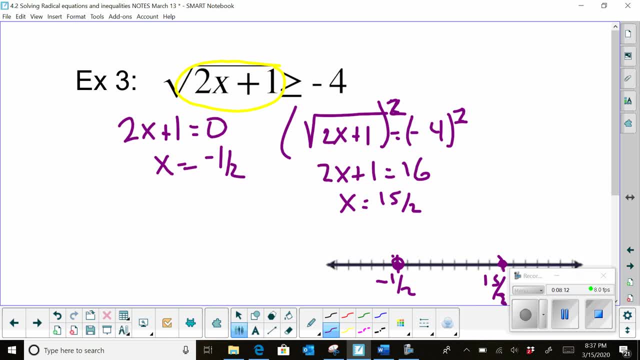 then let's test some values. We already knew that you can't be less than negative. 1 half That would be give you a negative under the radical. Let's plug in 0.. 0 is always a good thing to test. So you have the square root of 2 times 0 plus 1 is 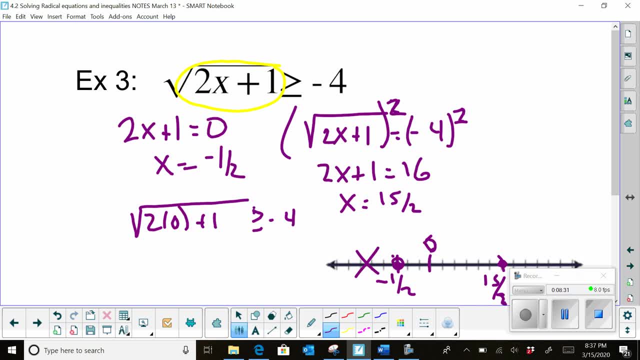 greater than or equal to negative 4.. When I do the square root of 2 times 0 plus 1,, that's just the square root of 1, which is 1.. Well, 1 is greater than negative 4.. So 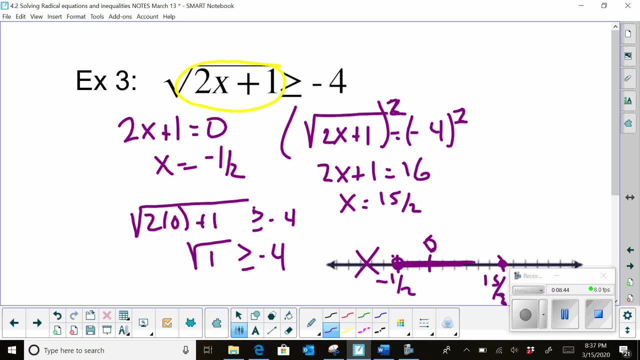 that's true. So I'm going to shade that. And then if I shade something greater than 15, halves like 8, 8 is going to work as well, because if I plug in 8, that's going to give me the square root of 2 times 8 plus 1 is. 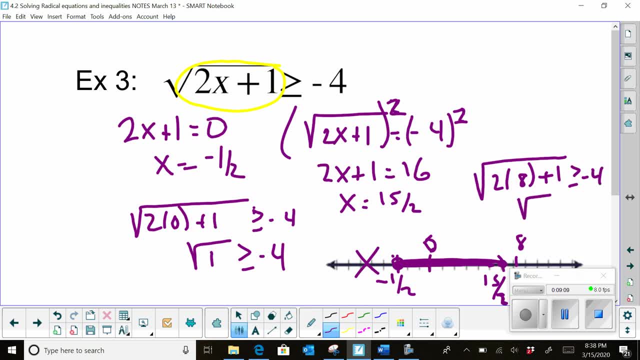 greater than or equal to negative 4.. And that's going to be the square root of 17,, which is definitely greater than or equal to negative 4.. So that works as well. What we have here is kind of an interesting thing, because we're going to have a square root of 2 times 8 plus. 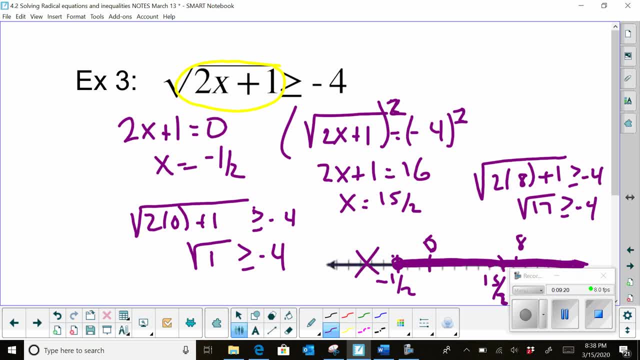 your number line continues through your closed circle. So we know that any value greater than or equal to negative 1 half would work in that inequality. So you're going to say the square root or, sorry, the closed circle, that's your bracket- negative 1 half to positive. 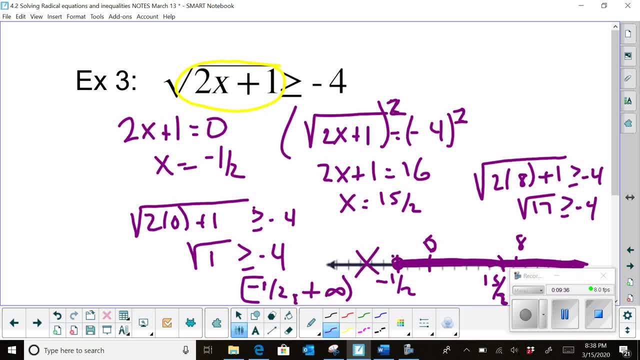 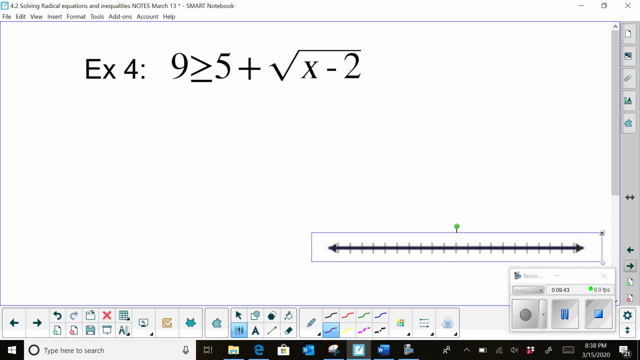 infinity. Again, I'll get the hang of this stylus soon. So we've seen some examples. Let's move on to the next one, This one. you're going to need to isolate your variable, your radical, Before you solve. But again, we always start with the radicand. It's like starting with 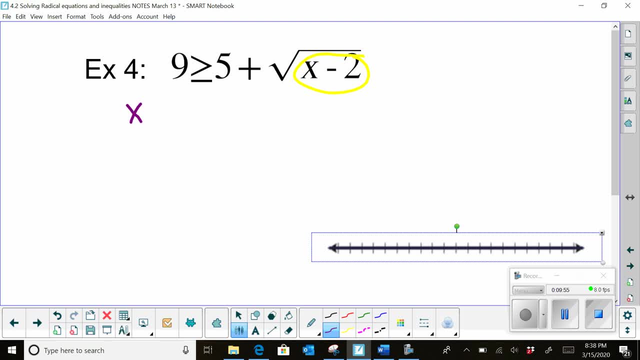 the denominator and the rationals- Remember those- couldn't equal 0. This time, x minus 2 equals 0. So you're going to say x equals 2.. So you know that 2 is going to be one of your circles. You'll put a closed circle at 2.. And I know that anything less than 2 is. 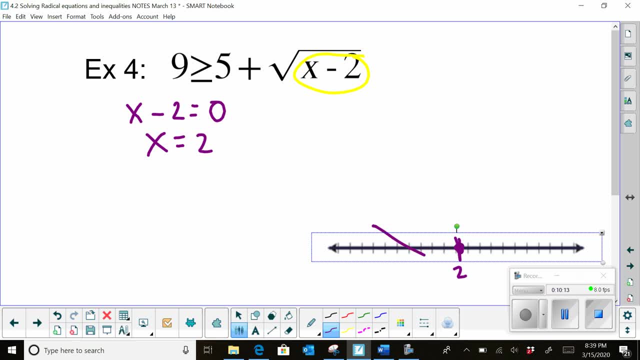 not going to check, because anything less than 2 would give me a negative under the radical. So you don't even have to check that part of the number line. It's not going to work. Then we're going to turn it into an equation: 9 equals 5 plus. 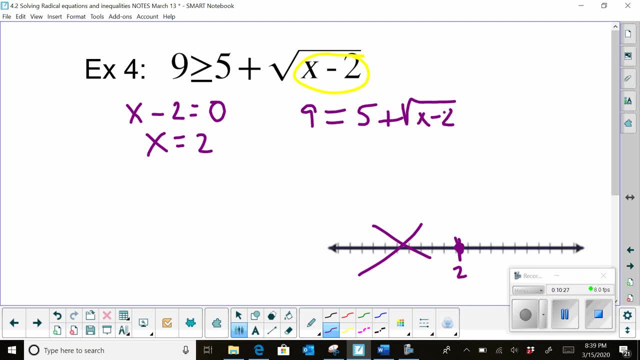 the square root of x minus 2.. You have to isolate your variable. So subtract 5 over first, You get 4 equals the square root of x minus 2.. You need to square both sides to isolate the variable. Get rid of that radical. So you get 16 equals x minus 2.. 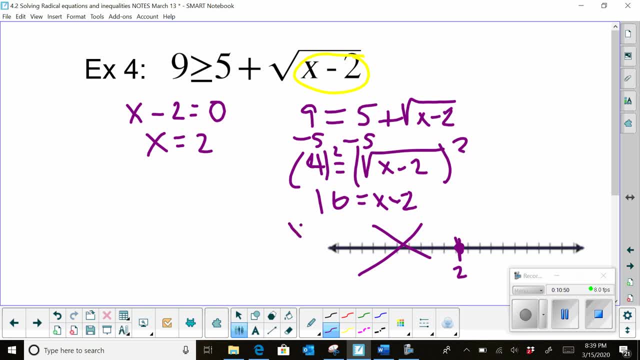 Add 2 to both sides and you get 18.. So 18 is our other circle. Again, that one will be closed as well. And then let's pick something easy to test between 2 and 18 like 3.. So we're going to plug in 3.. I'll come over to the side. 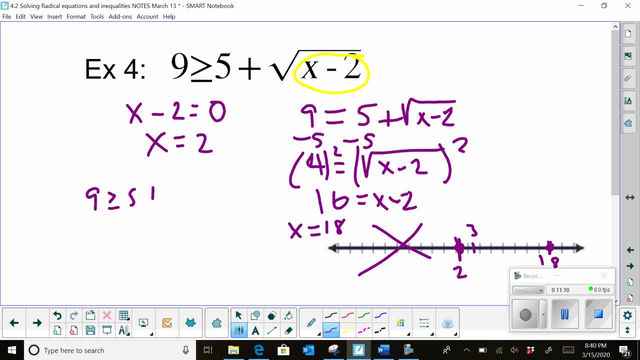 9 is greater than or equal to 5 plus the square root of 3 minus 2.. So that means 9 is greater than or equal to 5 plus the square root of 1, which is 6,, and 9 is greater than. 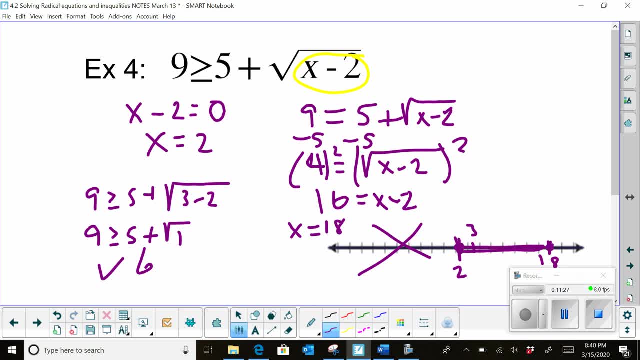 or equal to 6, so that's true. So we're going to shade between- I know that's going to work And let's try something beyond 18, like 19.. So we'll try 19. We're going to do. 9 is greater. 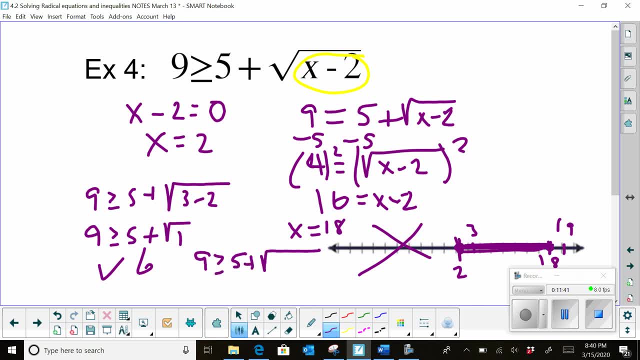 than or equal to 5 plus the square root of 19 minus 2.. Well, 19 minus 2 is what? 17?? And I know the square root of 17 is something slightly greater than 4, so 5 plus something. 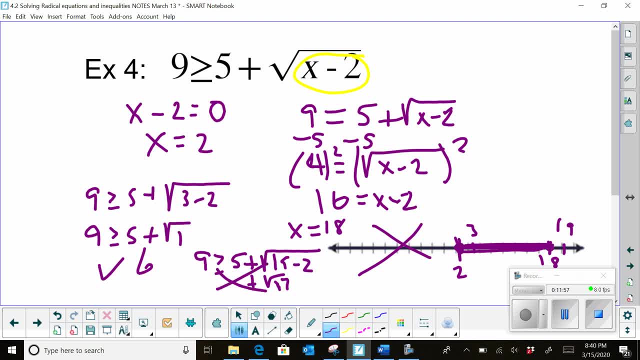 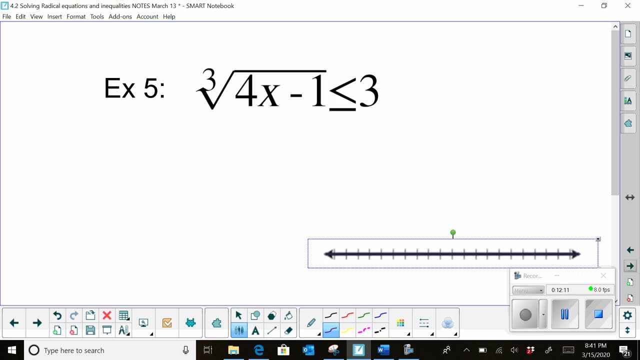 slightly greater than 4 would be greater than 9, so that does not check. So 19 does not check and our solution is going to be 2 to positive 18.. One more example, Let's try this one. It's a cube root, So again, in a cube root, anything can be. 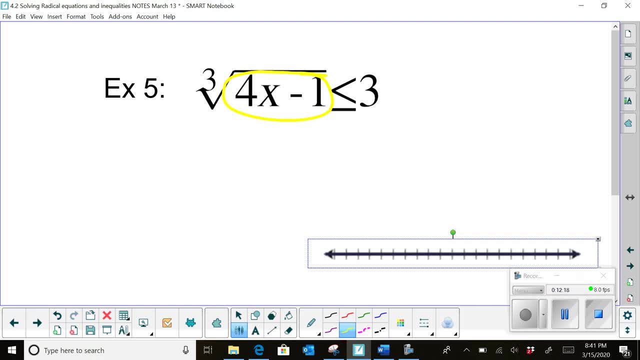 the radical can be anything positive or negative. So in a cube root you don't have to worry about a restriction under the radical because, remember, cube roots can be negative. It can be a positive or a negative. So this time we don't have to set the radicand equal to 0. You're just going to turn. 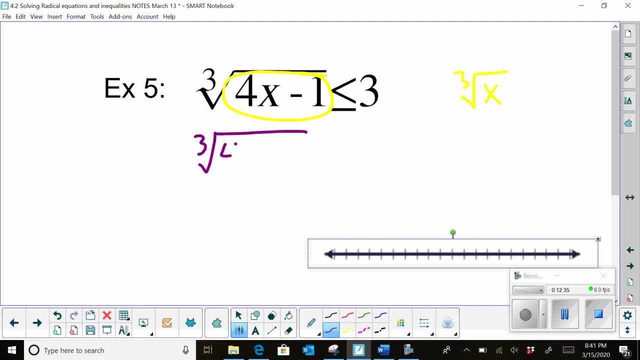 this into an equation and solve and then test your points. So you've got the cube root of 4x minus 1 equals 3.. We're going to cube both sides, because that's what undoes the cube root. You're going to take the square, the cube root, excuse me, and the cube we're. 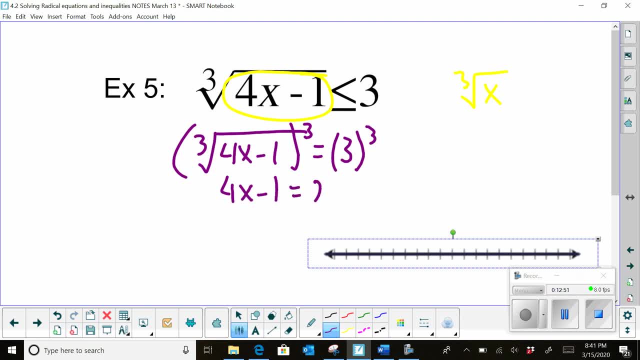 going to cancel out. You get: 4x minus 1 equals 27.. That's 3 cubed. So you're going to add 1 and divide by 4.. So x will equal 8.. No 7, sorry. And then you're going to plot that.